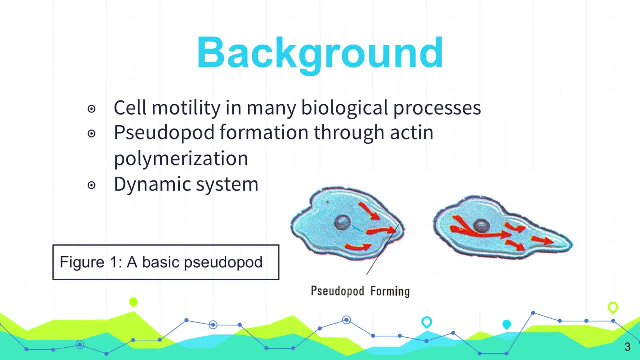 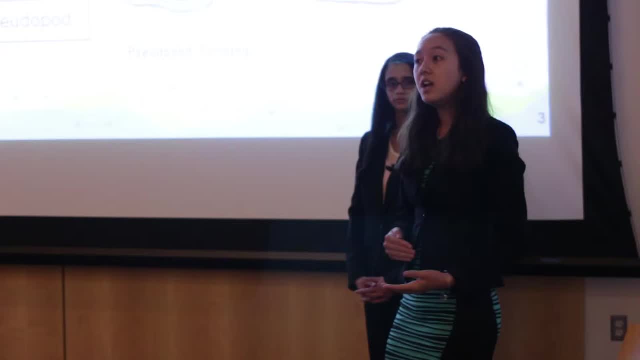 pushes outward on the membrane to perform a growth on the surface of the cell. Pseudopod formation is known as a dynamic system because it involves activators that are limited by inhibitors. Together, the activators and inhibitors regulate each other and can form many patterns. 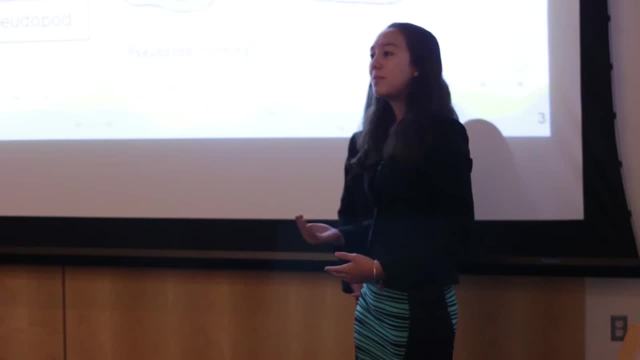 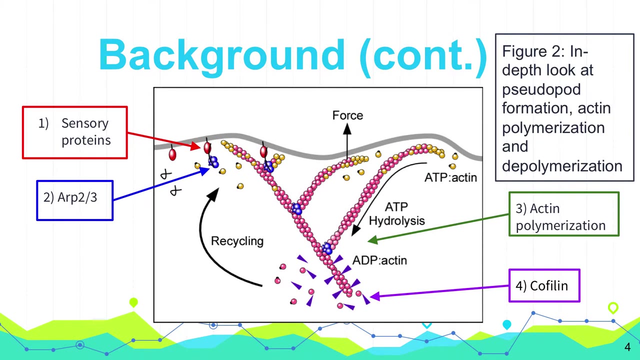 commonly found in nature, such as the unique stripes on a sishell or the strong red letter. This is a diagram of pseudopod formation through actin polymerization. First we will look. We have the sensory proteins which are indicated by a red arrow. 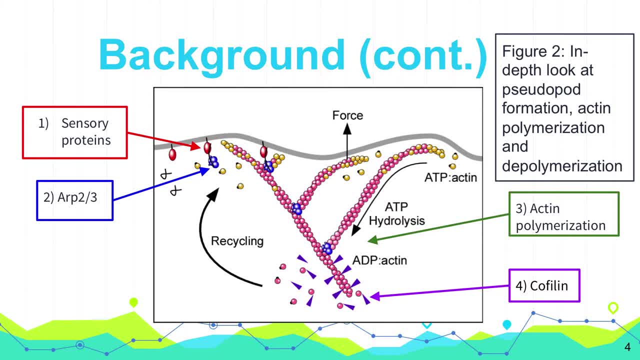 and these proteins detect chemical signals from the extracellular environment which is outside the cell. These proteins then trigger another protein, ARP2-3,, which is indicated by the blue arrow. ARP2-3 then initiates nucleation. During nucleation, one ARP2-3 protein combines with three actin monomers. 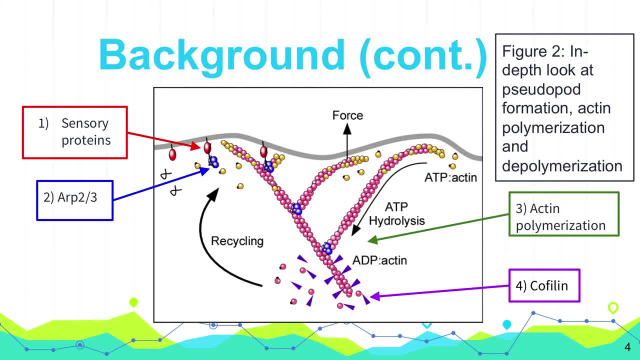 This complex then builds because more actin monomers build upon it and form a chain, also known as an actin filament. One actin filament cannot apply a large enough force to create a pseudopod, so more ARP2-3 proteins join onto the existing actin filament and branch off. 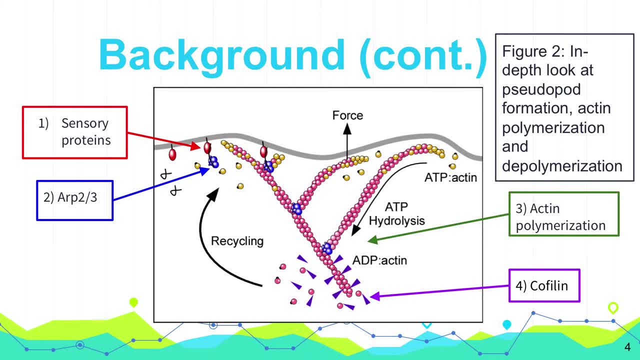 This network of actin can exert a force large enough to push the cell membrane and create a pseudopod. However, there is a limited amount of actin monomers In the cell, so the actin needs to be recycled. This is done by the protein cophalin, which is indicated by a purple arrow. 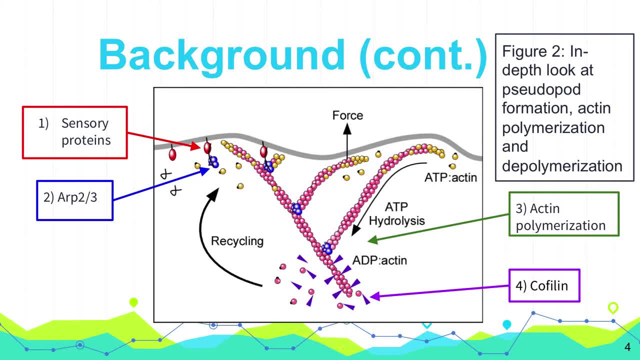 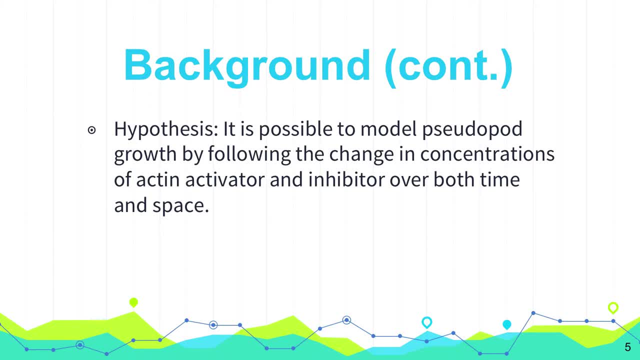 The cophalin removes some of the actin from the bottom of the filament, as you can see in the diagram, and releases the actin to be reused later. Our goal for this project was to virtually model pseudopod growth and we hypothesized that by translating algorithm that models the change in concentration of actin activators. 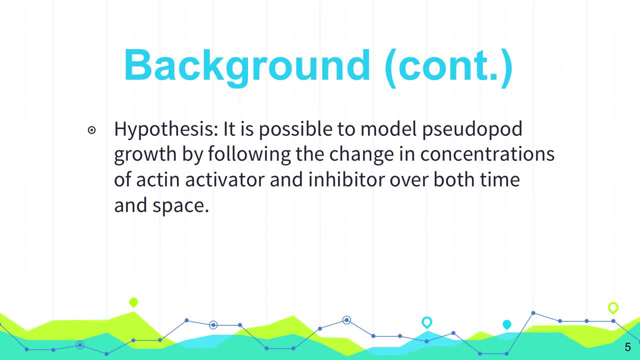 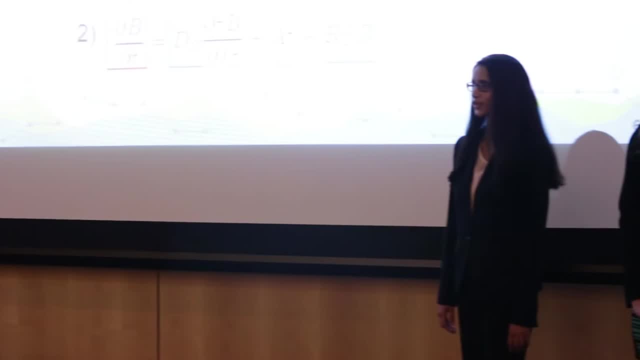 and inhibitors over time and space, we would be able to model pseudopod growth and cell motility. To begin our procedure, we tried modeling cell motility mathematically. In order to do this, we had to think of the cell as a dynamic system. 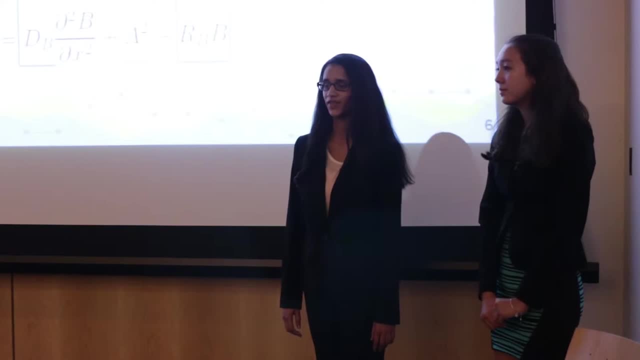 The protein ARP2-3 and the actin monomers were the activators because they promoted the growth of pseudopods. The protein cophalin was an inhibitor because it slowed down the growth. Here we have two coupled partial nonlinear differentials. 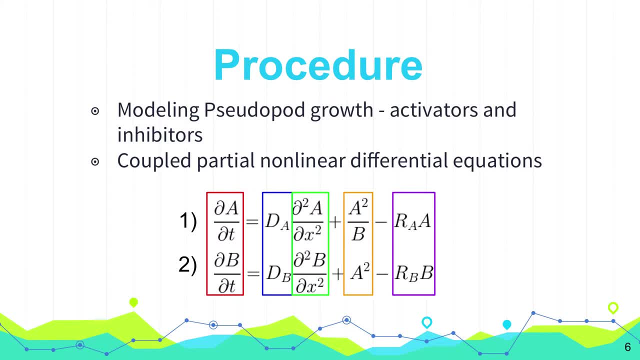 The first one describes the activator, which is denoted by the letter A, and the second one describes the inhibitor, which is denoted by the letter B. These equations particularly use derivatives, which are basically the slope or the rate of change of something. 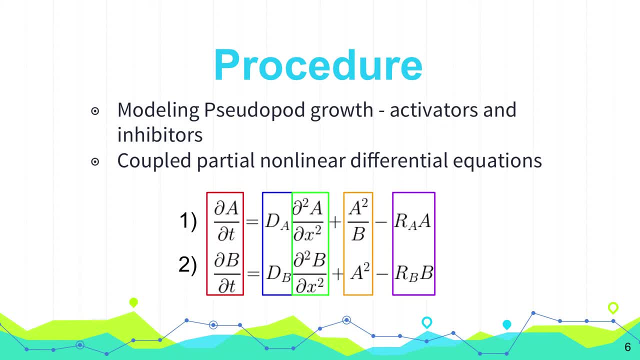 In our first equation, the first term is partial A over partial T, or the rate of change of the activator with respect to time. The next term, which is boxed in blue, is dA, which is the diffusion coefficient, which basically indicates how quickly the activator diffuses. 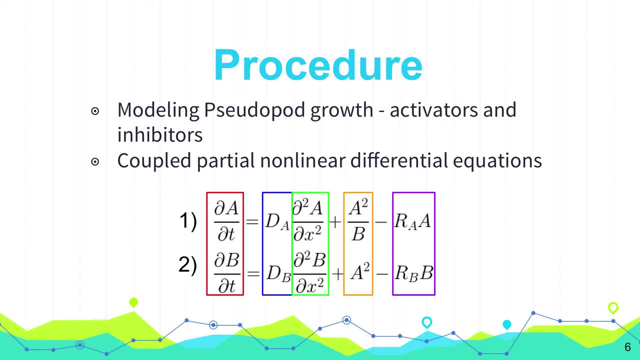 The next term, boxed in green, is the second partial derivative of the activator with respect to space. Next we have A squared over B, which is boxed in yellow, And A squared accounts for the branching mechanism of the actin, and this is divided by B, the inhibitor, because the inhibitor slows this down. 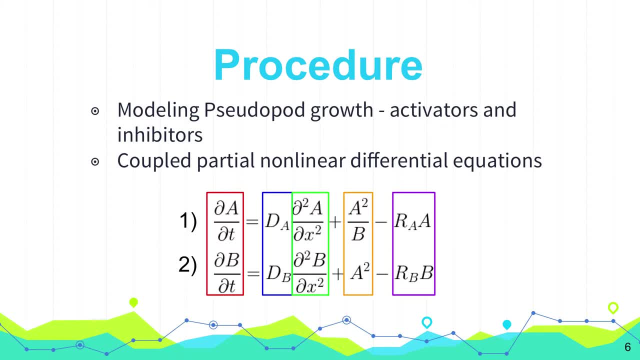 And then in blue we have RA times A, and RA is the rate of change of the activator with respect to time, and RA is the rate of change of the activator with respect to time, and RA is the rate of change of the activator with respect to time. 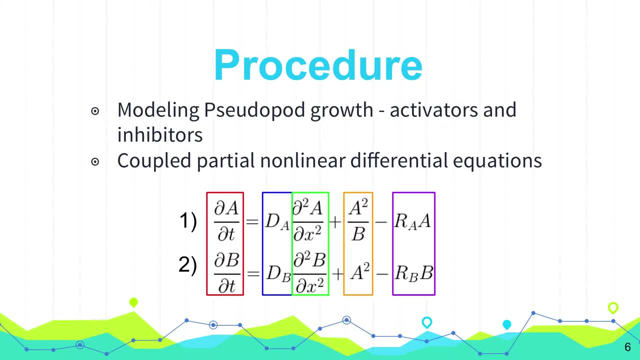 And RA is the reaction rate of decay of the activator. So this term is subtracted because, as the activator decays, obviously the system would slow down. The second equation is similar to the first equation except, as you can see, A squared is not divided by anything. 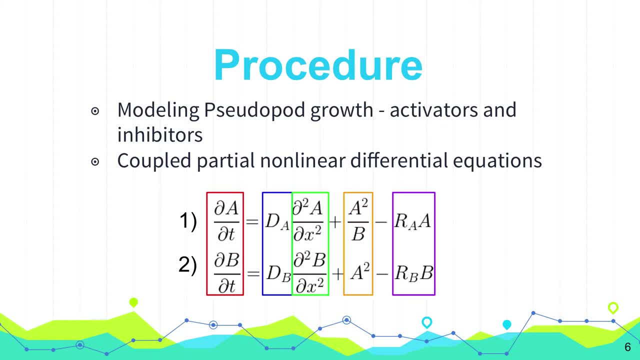 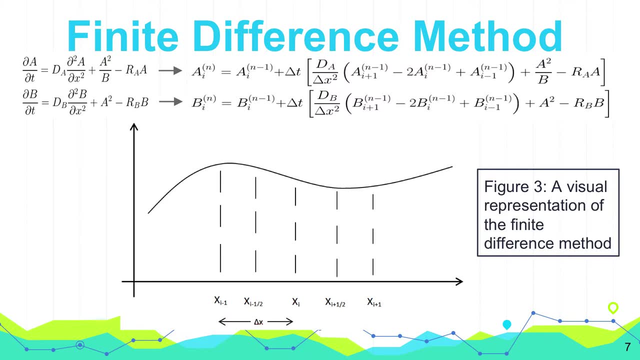 This is because there's nothing to slow down the inhibitor. Using the finite difference method, we can take these differential equations and translate them into algebraic expressions which can then be analyzed numerically using the program MATLAB. The finite difference method involves using discrete points in space. 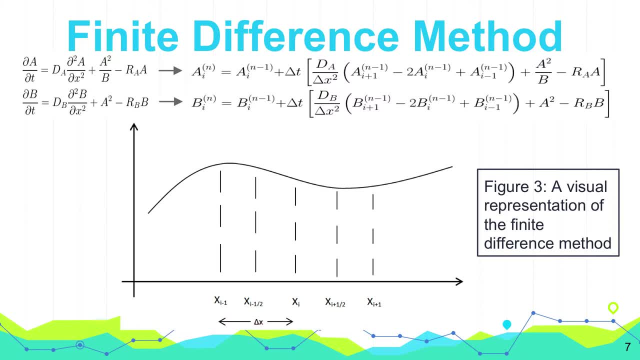 such as xi, xi plus 1, and xi minus 1,, all evenly spaced out by delta x. By taking the derivatives at these points, we can translate this equation on the left into the equation on the right. On the right hand side, n is not an exponent but rather an index for time. 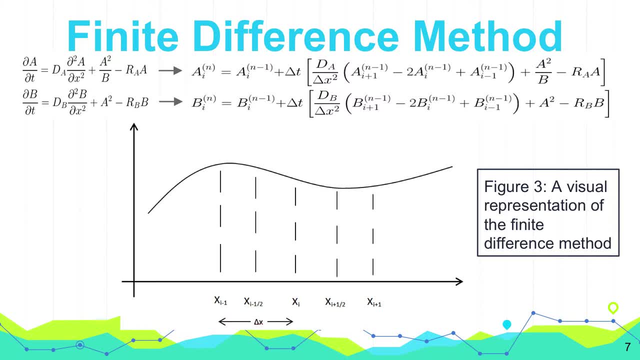 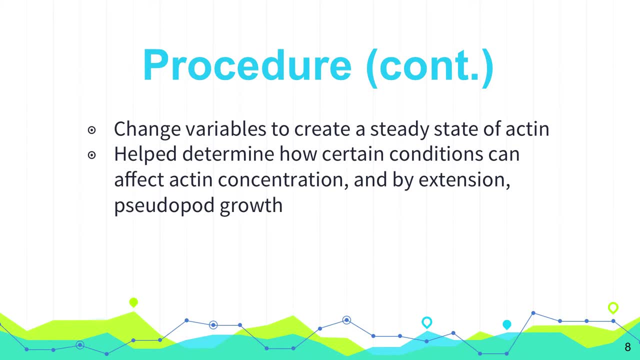 while i is an index for space. This equation on the right can then be plugged into a program such as MATLAB. Once we have our equations programmed into MATLAB, we can use our knowledge of dynamic systems in order to change certain variables, such as the diffusion and reaction rates. 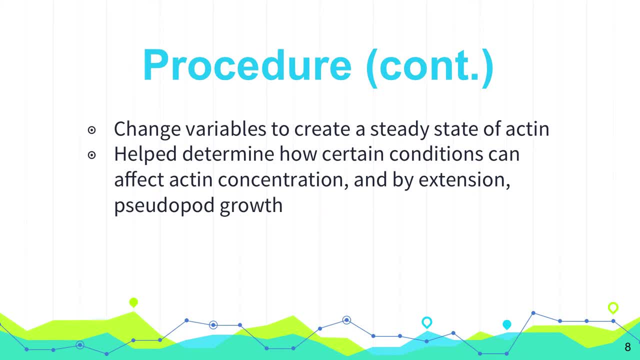 We were trying to achieve a steady state of active concentration, which would represent a constant presence of pseudopods within the cell. The purpose of these experimental changes was to try and determine how certain variables or conditions within the cell would affect pseudopod growth. 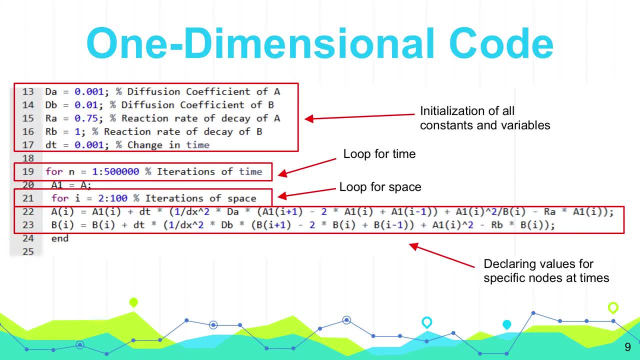 The following image is a portion of our one-dimensional code, which allowed us to understand how different parameters affected the pseudopod growth. As you can see in the beginning, there are several variables that allow us to manipulate this growth Afterwards. we have two for loops. 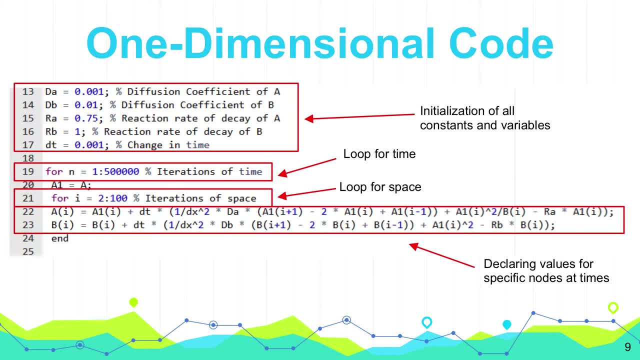 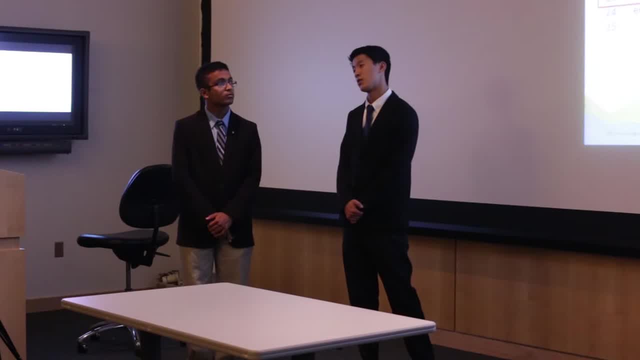 The beginning is the n for loop, which allows us to account for time, and the second one is the for loop for i, which accounts for space. By plugging these two equations within these two loops, we can then calculate the concentration of both. a the activator. 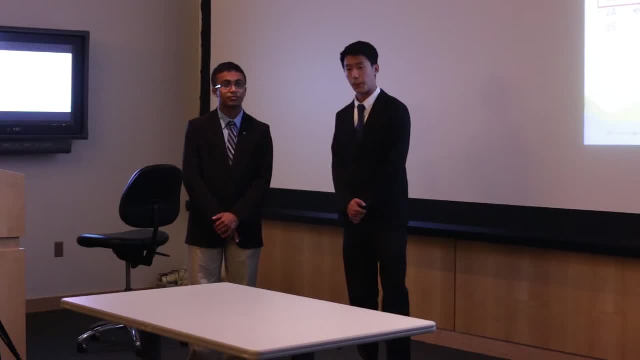 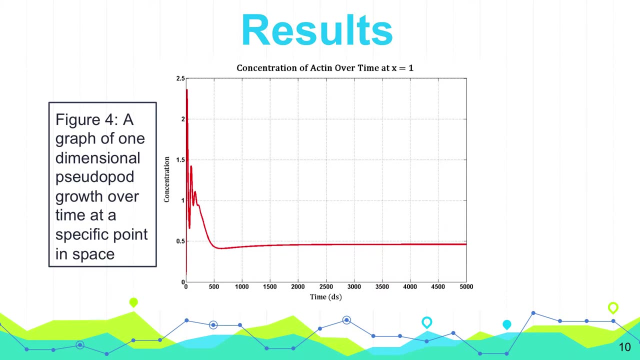 and b the inhibitor at a location in space and time. This is the result of the following code: This plot is the concentration of acting over time at a specific location in space. in this case, x equals 1.. After initial fluctuations in the concentration. 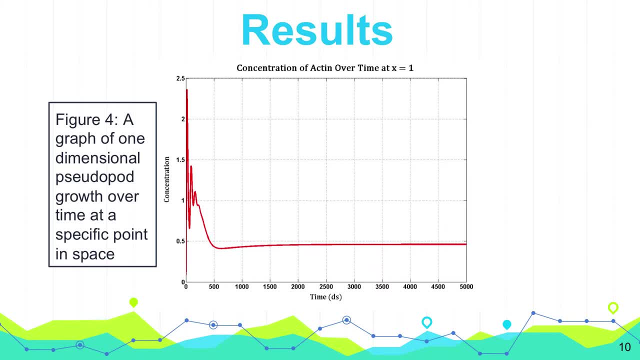 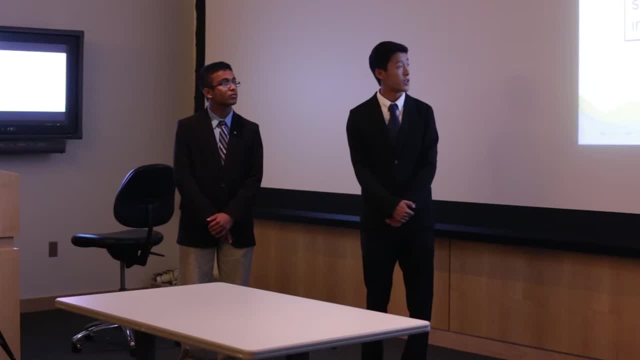 we can see that the line steadies out into a horizontal line. This horizontal line represents the steady-state equilibrium between the activators and the inhibitors, which allows for constant pseudopod existence. If, for instance, the line were to instead decrease to zero. 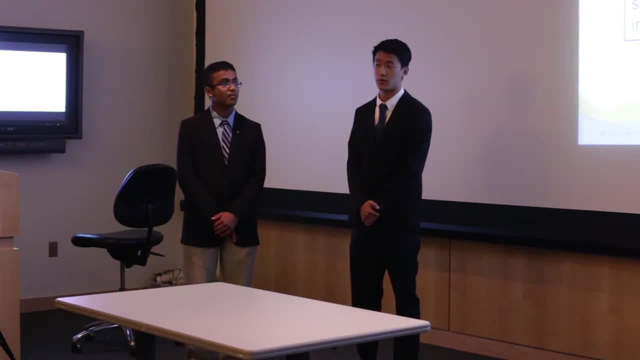 the inhibitors would have overtaken the activators and the pseudopod would not be able to grow. Likewise, if the line were to increase to infinity, the pseudopod would grow limitlessly, which is not efficient for the cell. Here we have a table detailing the effects. 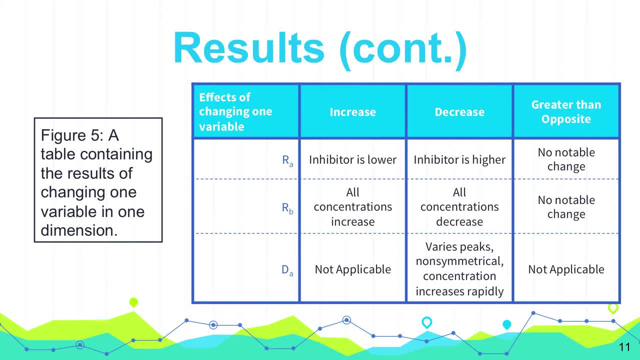 of changing a particular variable on a result. For example, if we increase the value for rA, we saw that the concentration of the inhibitor decreased. Also, if we decrease the value for rA, we saw that the concentration of the inhibitor increased. 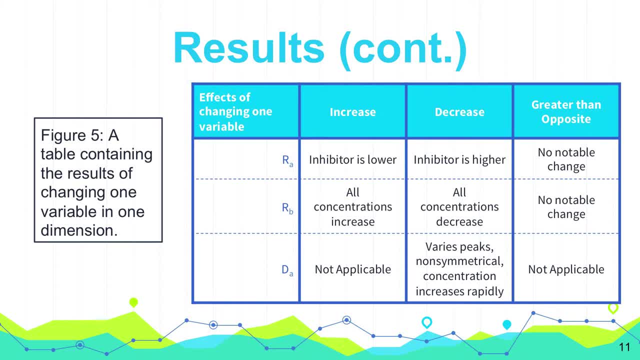 We also wanted to see if there was any inherent relationship between rA and rB. so we tested to see what happens when we increase the value of rA above rB And we saw that there was no notable difference and there was no notable change. 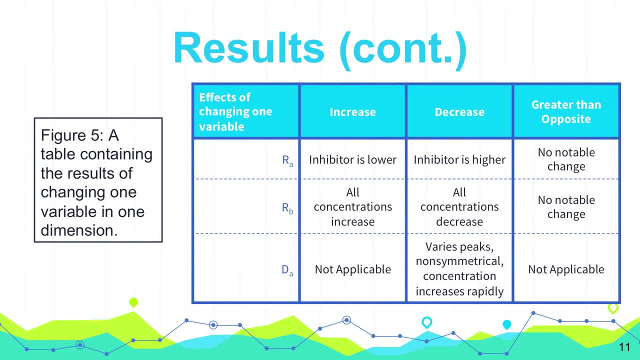 indicating that there wasn't any relationship between the two. We also changed the value for rB, and when we increased it, we saw that all concentrations of activators and inhibitors increased. Likewise, when we decreased the value for rB, we saw that the concentrations of activators and inhibitors decreased. 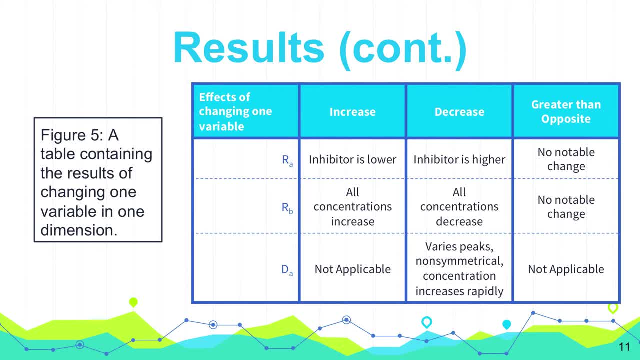 Finally, we tested for dA. We did not increase the diffusion coefficient, because by increasing this, we would enable the activator to diffuse more quickly, which would prevent a pseudopod from forming at all, which is not what we wanted. 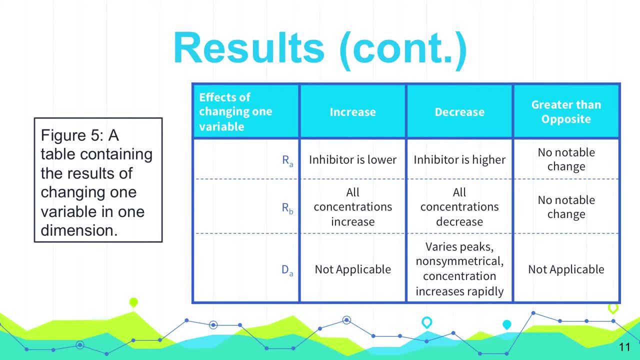 Therefore, we only tested by decreasing the value of rA. Thus, when we tested this, we saw that there was a varied number of peaks, which indicates numerous pseudopods forming, and we also saw that they were non-symmetrical. 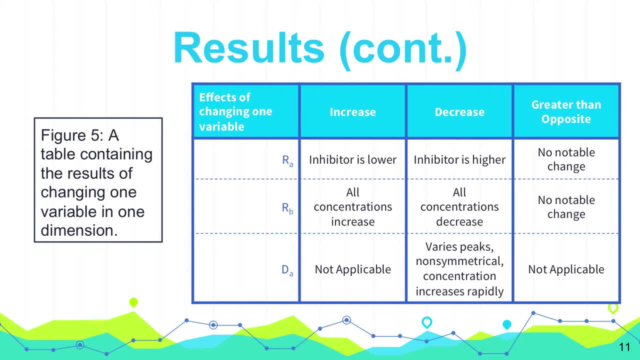 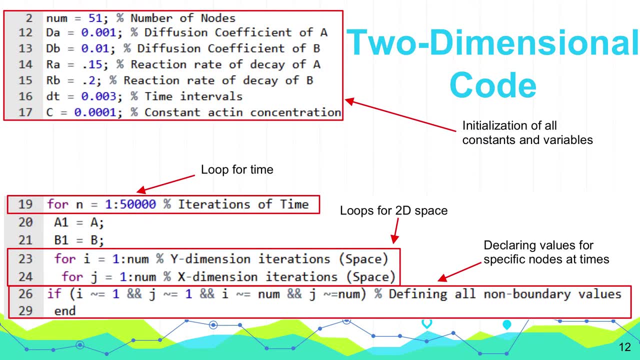 which indicates a random nature in the time at which they formed. Finally, we saw that the concentrations of actin activators and inhibitors increased rapidly. Here we have the sample of our final two-dimensional code. In the top we have an initialization of all constants and variables. 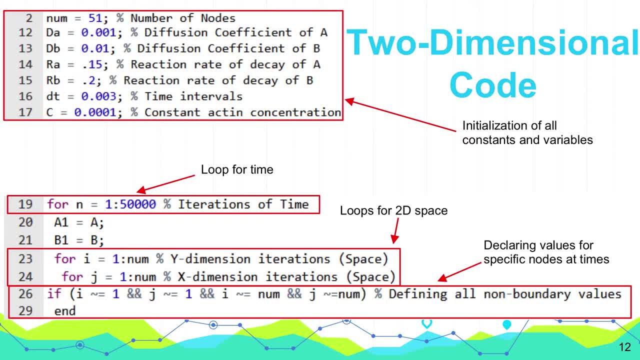 At the very top, you see that num equals 51. This is the number of nodes in space. Because it is two-dimensional, it's a 51 by 51 matrix of different points in space. Next, we have three different loops, the first being a loop for time. 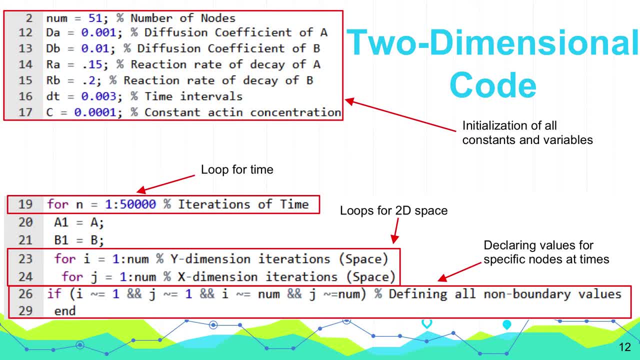 This loop consists of 50,000 iterations of time, which we measured in deciseconds for our scenario. Secondly, we have two different loops for space, the first being for the y dimension and the second for the x dimension. Finally, we declare values at specific nodes at specific times. 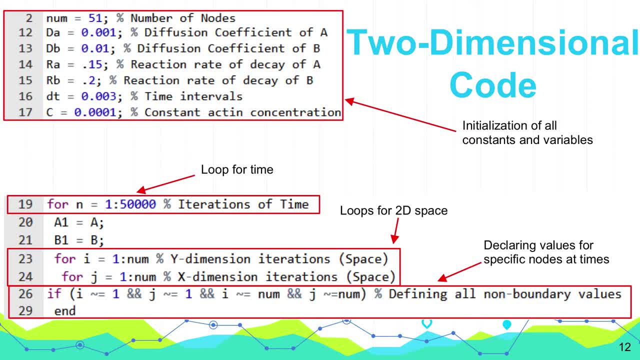 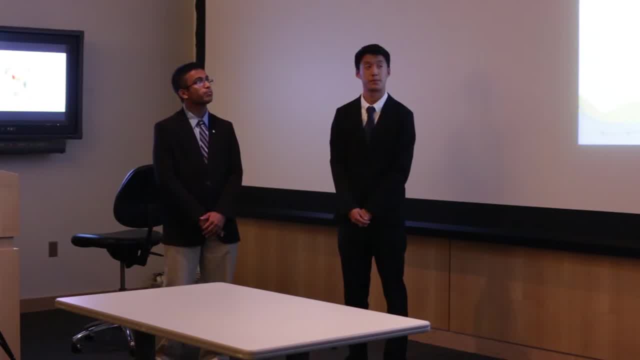 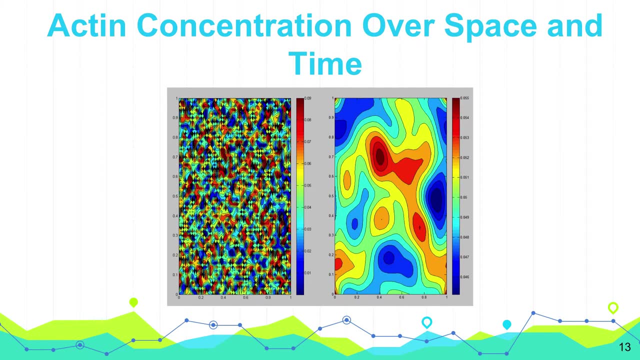 depending on their location in space. For example, here we defined all non-boundary values. We also defined boundary values and corner values separately. This image represents two-dimensional pseudopod growth over space and time. In the first image you can see the colors are all very random. 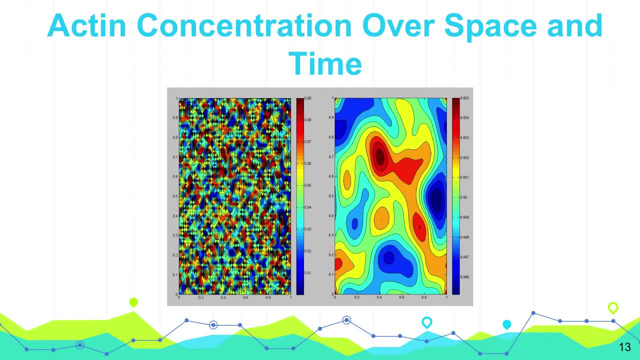 and that's because the cell is receiving a lot of random signals from another environment. Over time the active concentrations within the cell will diffuse and, as you can see in the second image, the dark red areas are where the active is most highly concentrated. 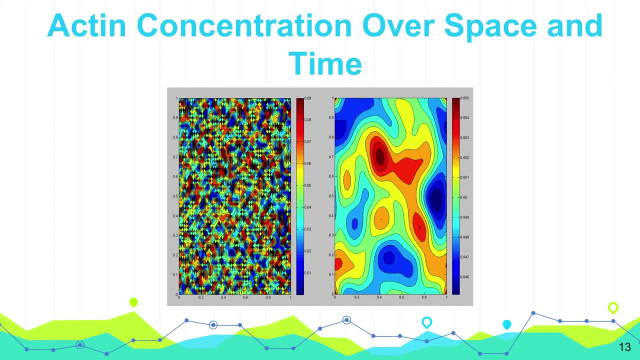 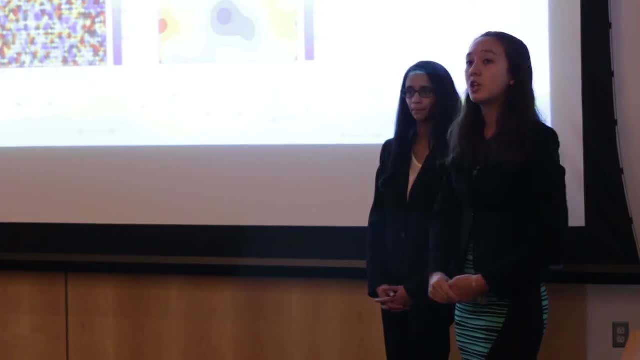 These are where a pseudopod would have formed. Now, because the active concentrations have diffused, the red areas in the second image are not as concentrated as the red areas in the first image, which is noted by the color bars inside each image. 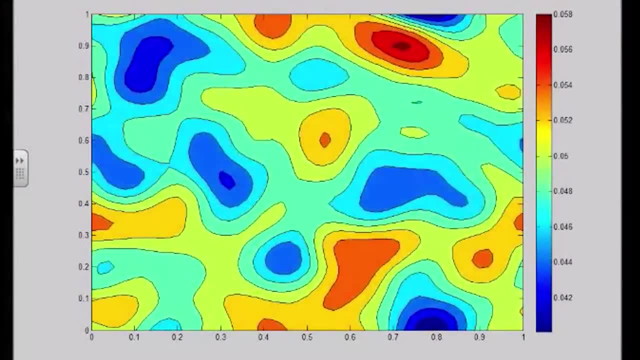 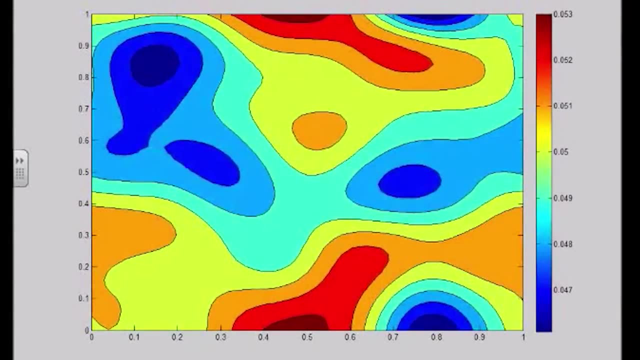 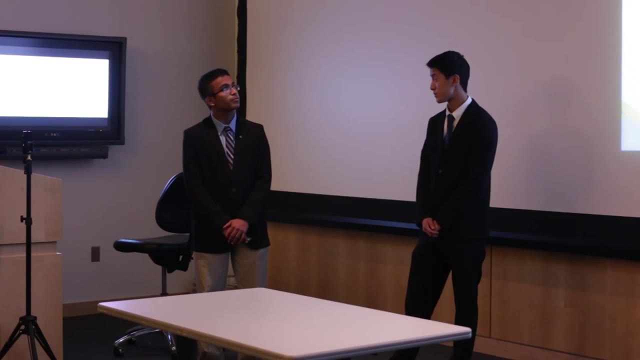 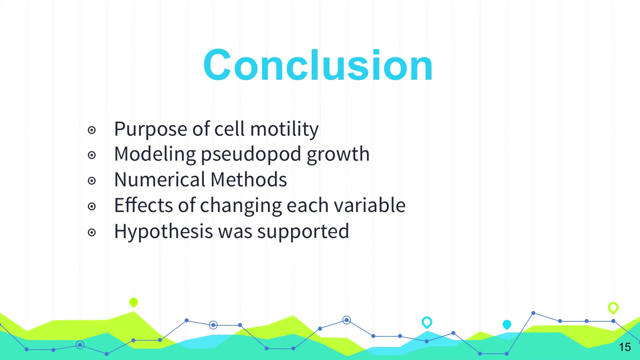 This is an animation of the following model. Notice how the concentrations slowly diffuse out and all objects of high concentration remain, indicating likely pseudopod existence. To recap, cell motility is important to most biological processes. In our project, we were able to model pseudopod growth. 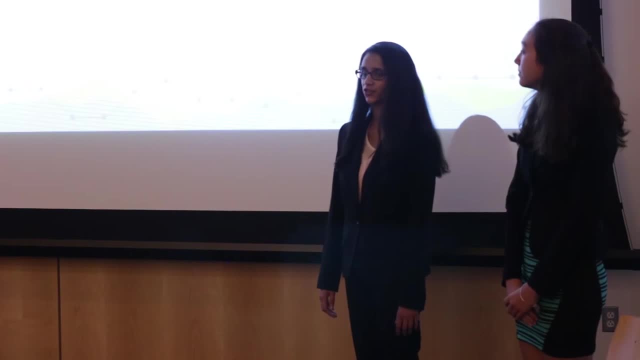 using MATLAB, a computer program. We did this by starting with equations and then using the finite difference method, a type of numerical method, to simplify them so they could be solved by a computer. We examined the effects of changing each variable in one dimension. 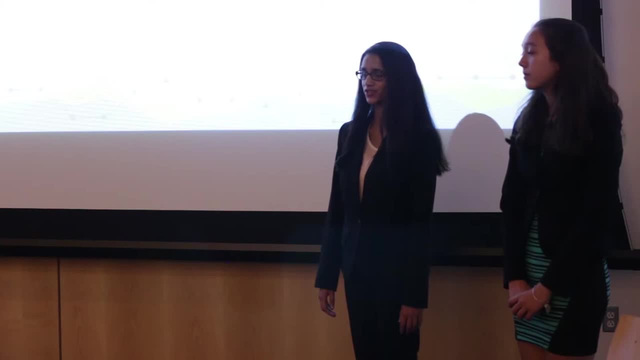 and noted that changing the reaction rates changed the concentrations, while changing the diffusion coefficient changed the nature of the peaks. We were also able to extend this into a two-dimensional model. as you can see in our animation, Our hypothesis was supported because we were able to model pseudopod growth using a computer. 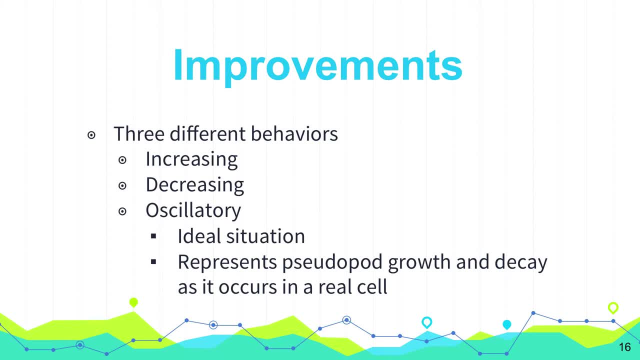 If we were continuing, If we were to continue working on this project, we would further manipulate the variables in order to achieve three separate graph behaviors. In our study, we were able to find conditions that led to increasing active concentration and decreasing active concentration. 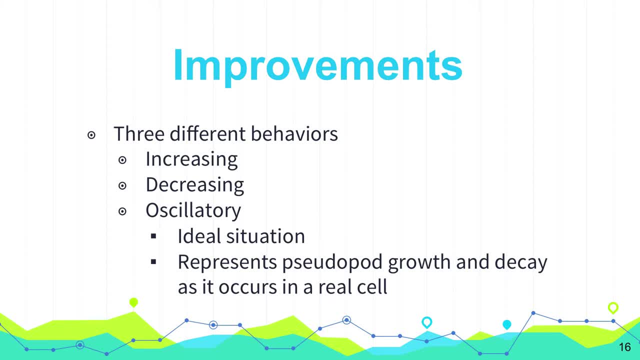 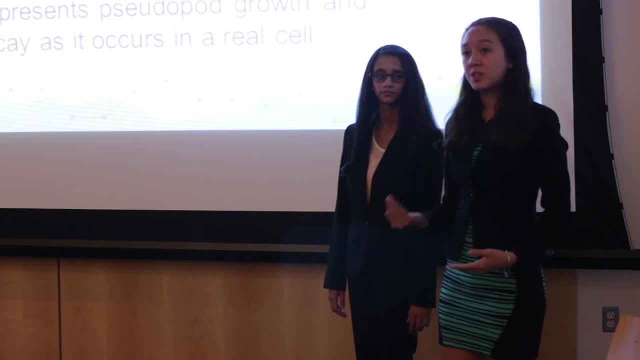 But in the future we would like to achieve an oscillatory active concentration. This is the ideal situation because it best represents conditions within a real cell. By better understanding how certain conditions within the cell affect pseudopod growth, we would be able to model the cell more effectively. 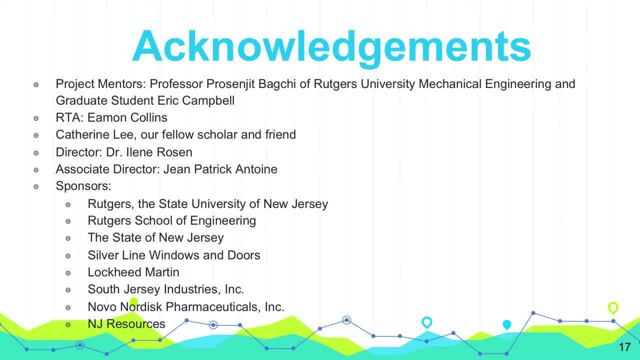 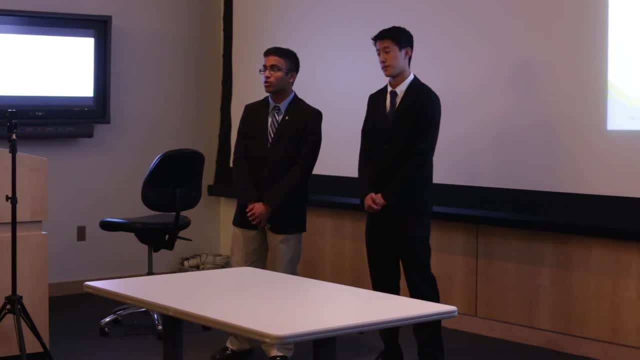 We would like to thank our mentors, Professor Sanjee Thakji and graduate student Eric Campbell, for their guidance and support for this project. We would also like to thank our RTA, Eamon Collins, as well as all the other RTAs that made this project possible. 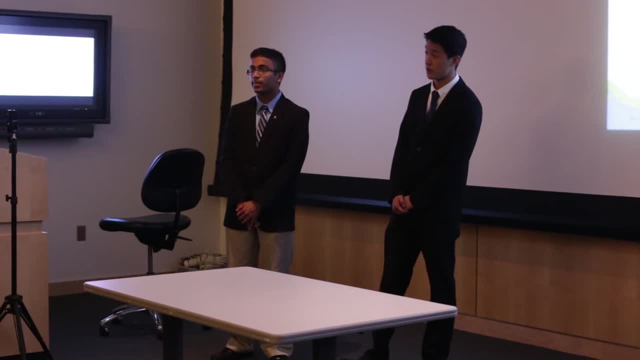 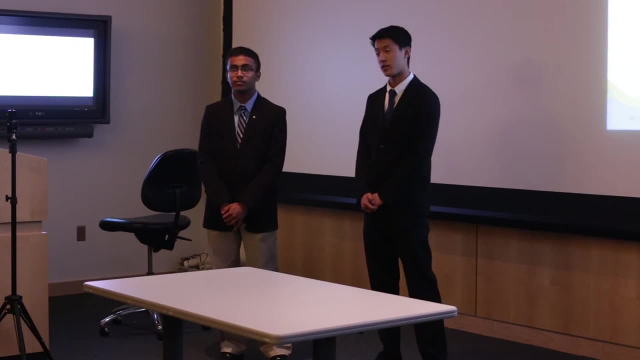 Additionally, we would like to thank Director Eileen Rosen and Associate Director John Patrick Antoine for conducting this program. We also want to thank Catherine Lee, our fellow friend and scholar. Finally, we would like to thank all the sponsors who can make this program possible. 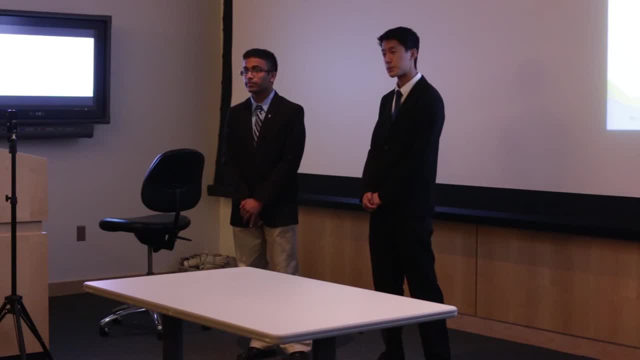 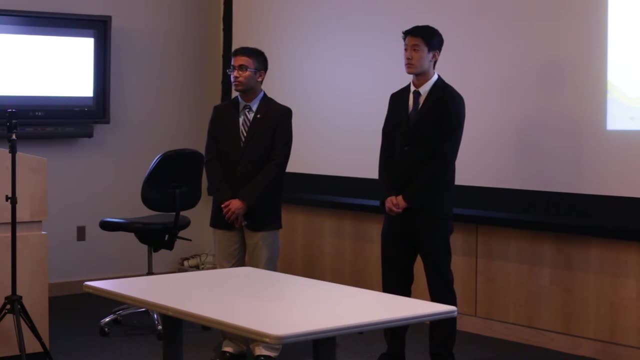 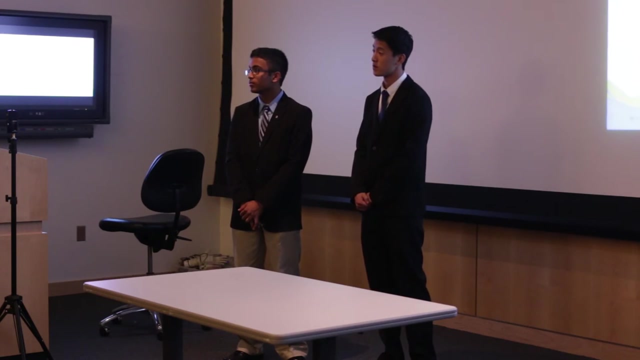 Thank you. Do we have any questions? Thank you, Are there any questions? Yes, Here you see, you're using the computing model, the kind of model of motion. Do you have any real data supporting comparing the coefficients coming from the real experiment data? 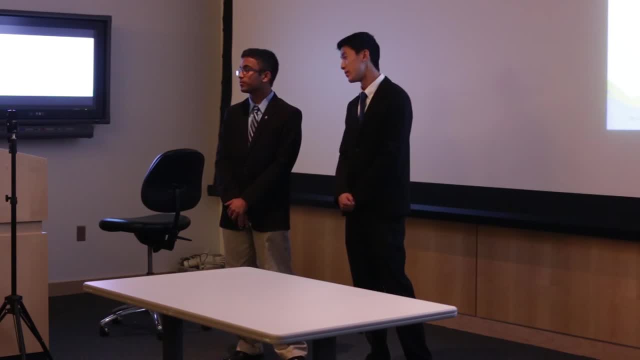 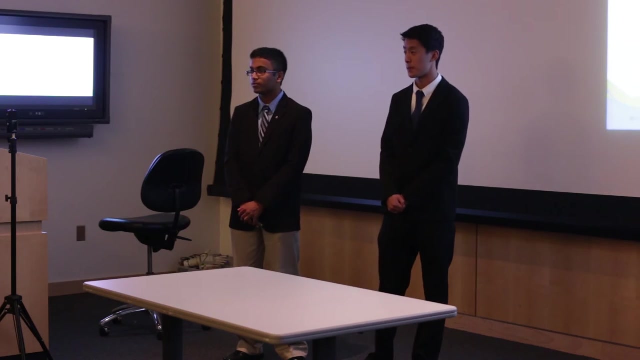 Did you repeat that? actually? Yes, This is a computing model simulation. Do you have any real data comparing with the real process? We were not able to actually take physical cells and analyze them ourselves. We only worked using computers at this project. Can you elaborate a little bit further on the significance of the student body formation? 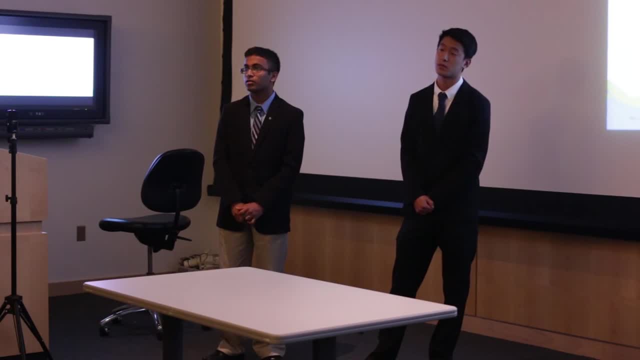 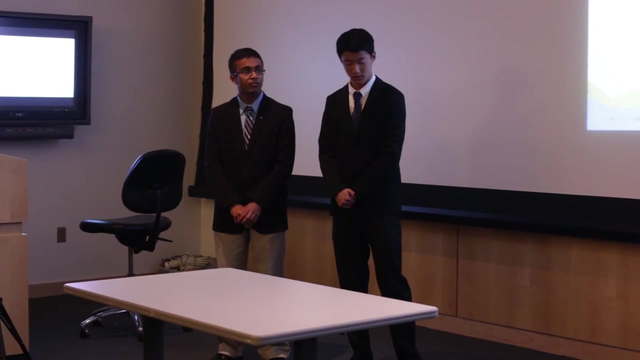 I assume at some point the idea is to change it or increase it or whatever, for maybe something like cancer treatment. Well, actually, cancer cells use pseudopods sometimes to metastasize and this is how cancer can come deathly in a lot of people. 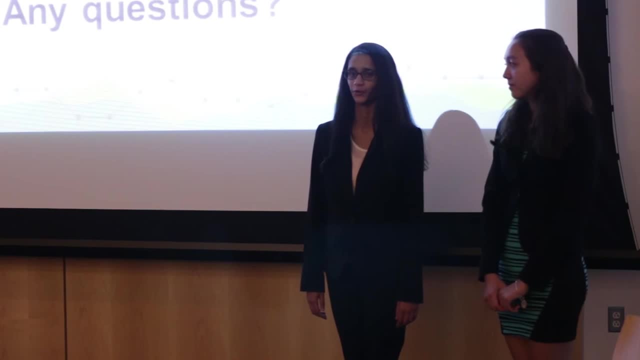 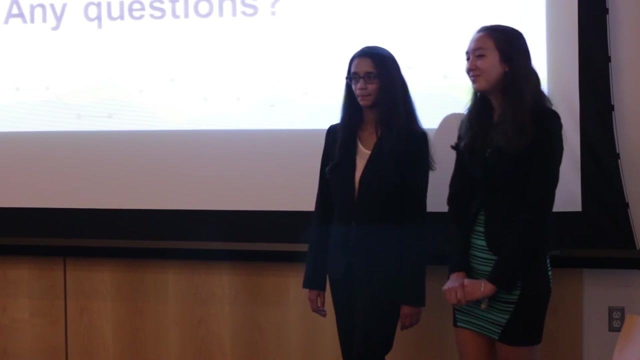 So by understanding cell motility and pseudopod growth. if one day we're able to come up with a way to slow down pseudopod growth, this could be applied to cancer treatment and slowing down the metastasis of cancer. I think there was a question on the phone. 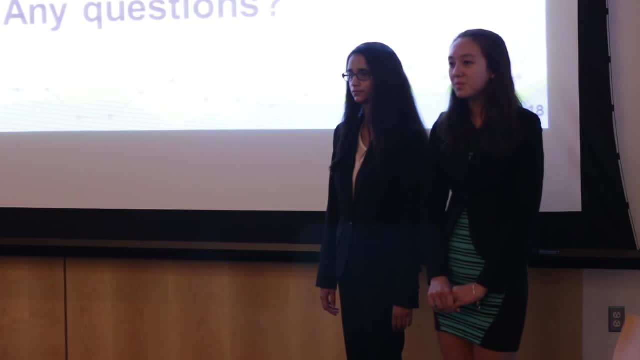 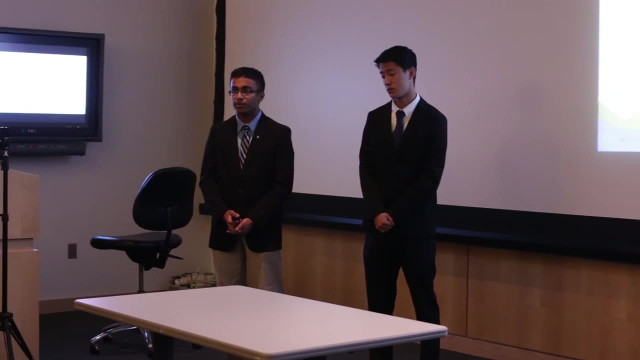 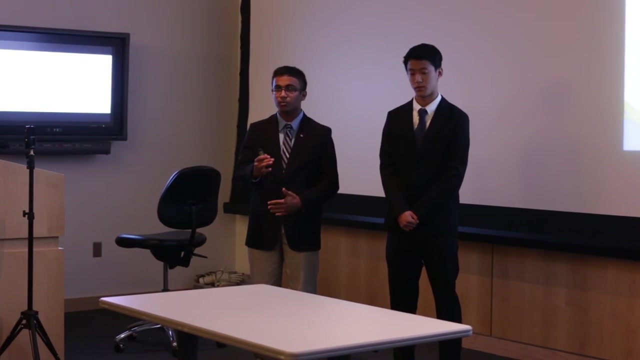 Can you tell us some of the challenges you faced while doing the project? I think the most difficult was the changing of the constants. There was a lot of different scenarios. First we had to individually analyze the constants, but then we had to play with them all together. 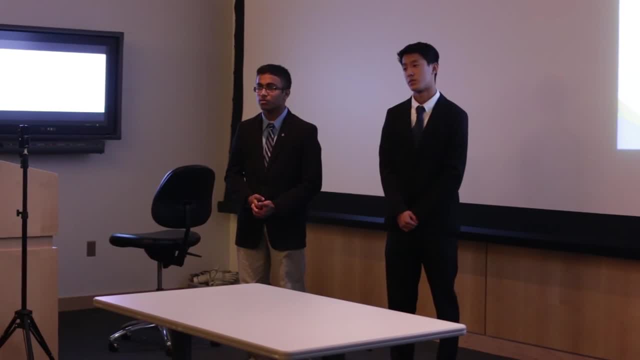 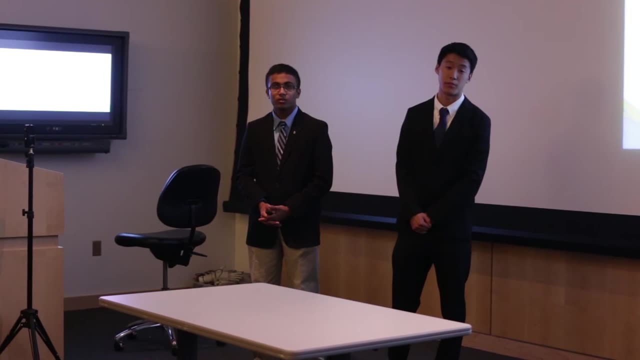 So there's a lot of different scenarios in terms of what their values can be. In addition, just the sheer time it takes to run one program with a set number of constants can take up to an hour because of the sheer number of iterations of time we're doing. 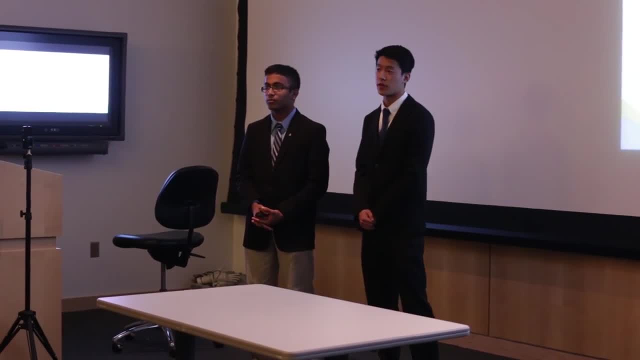 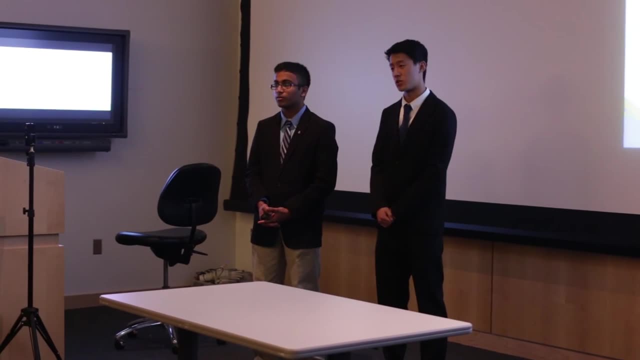 As we mentioned, we did 500,000 iterations, which takes a very long time. So running the entire set of code for like an hour and then analyzing that and then switching the code and running a new set for another hour takes a very long time. 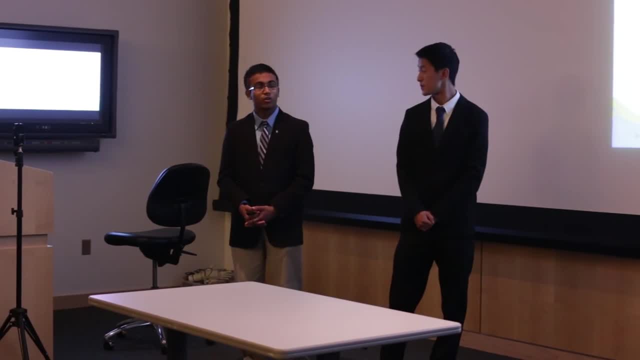 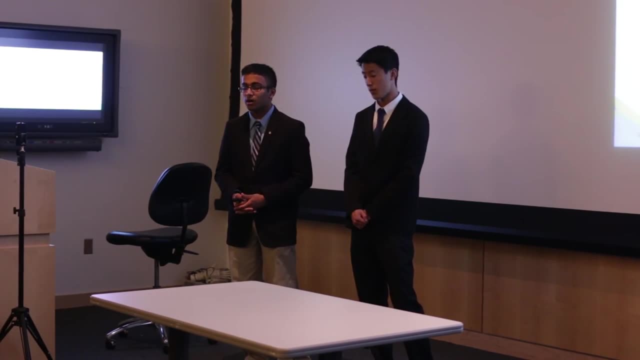 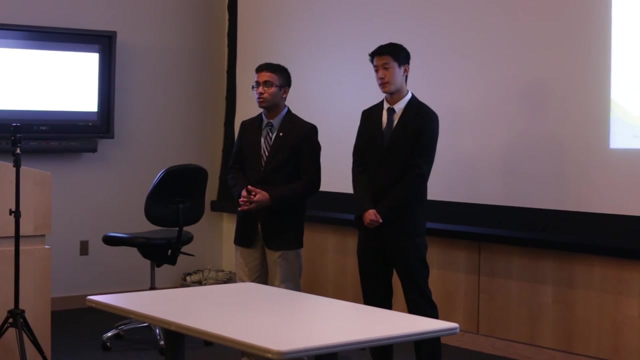 So that was definitely the hardest process And also in our project we have 51 different nodes, a 51 by 51 area, whereas an actual cell. we would want to be more accurate and model that with close to a million by a million different nodes.